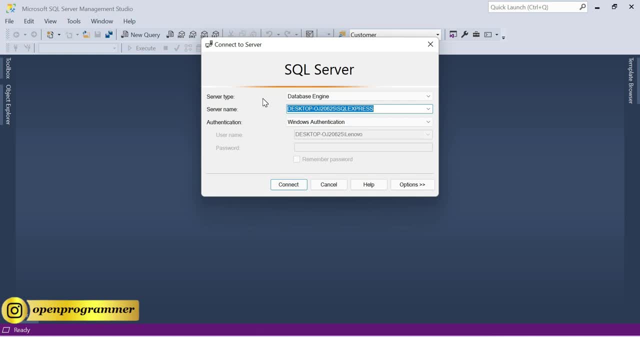 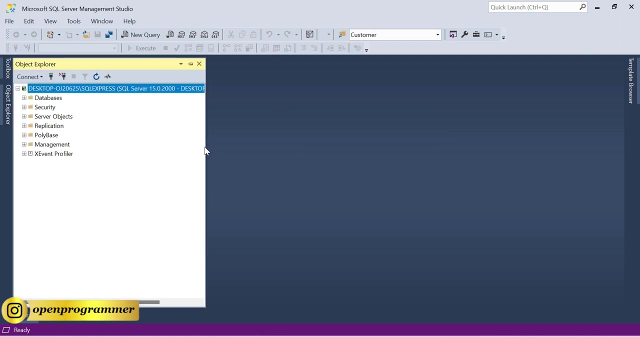 and download and install that sql in your machine. so this is my local server name: dextro-this slash sql express. so for your machine it should be a different name. so select your server name and click on connect so it will connect your local server. as you can see on screen, this is your object: explorer it. 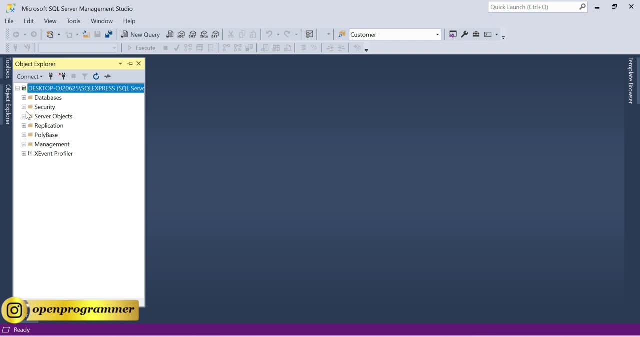 contains all the database list, login and other features. so if i expand this databases, so it shows me all the system databases as well as whatever i have created so far. so if you expand this, so these are pre-installed databases which are system databases and these are i have created. 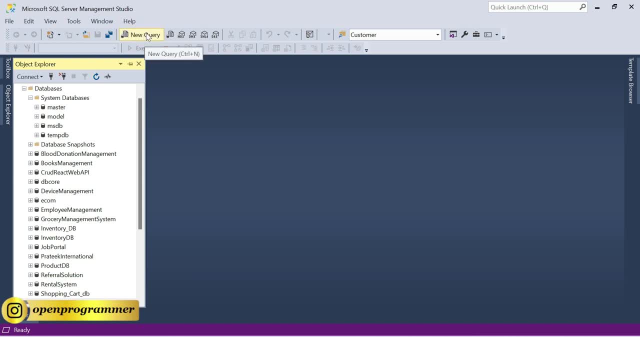 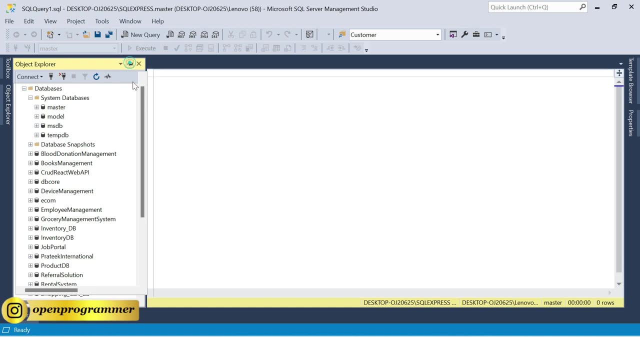 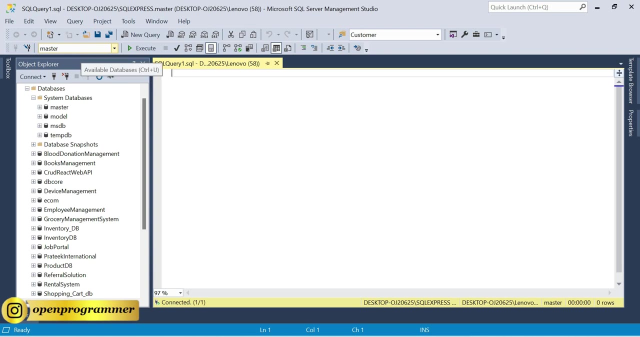 manually. all right now. you can see there is a button, new query. click on it so it opens a new query window. so here, once you click on this new query, it directly: uh, take microsoft- uh, sorry, master- as a default database. if you want, you can create a new database, but for this particular video i'm using 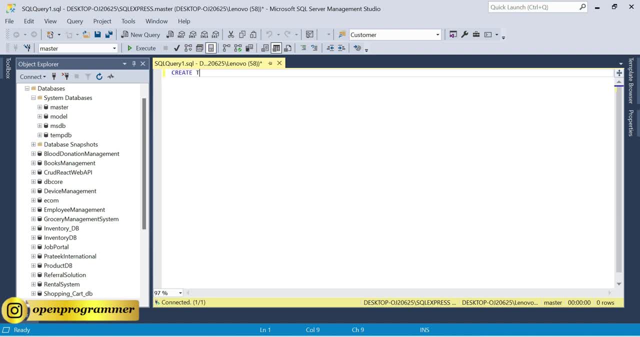 this master. so let's quickly create a new table. so let's say, create table crud stored procedure. i'm using a random name, so identity and that is primary key name: worker, agent, agent, agent, agent, agent agent Addresses where care, So the command, so you can see command completed successfully if I try to select the columns: select star from. 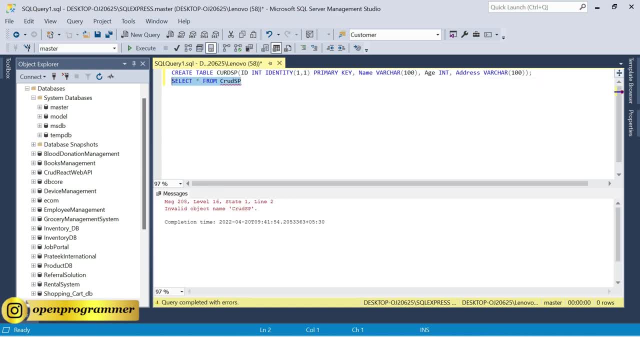 Crud SP. Oops, I misspelled the name, but anyways. So You can see ID, name, age and address. so for this particular table will create a stored procedure and perform all the operations. So to create a stored procedure, the command is create procedure and The procedure name. so there are two keywords: one is complete procedure and another one is proc, PR OC. 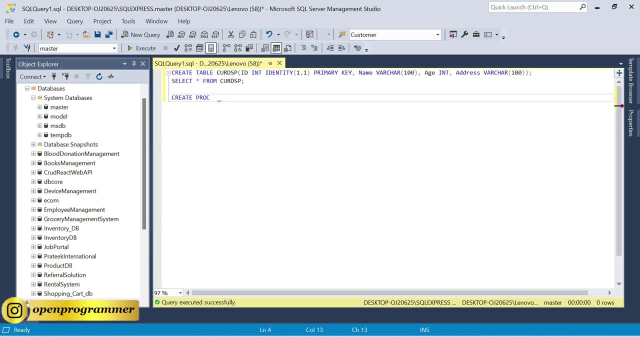 So either one you can use, so that is a shorter form, So we'll use Proc, so create proc and then the procedure name, so USP, Let's say employee Management, Has Begin and end, so this is the outer body of stored procedure. So in this particular video we are going to perform: 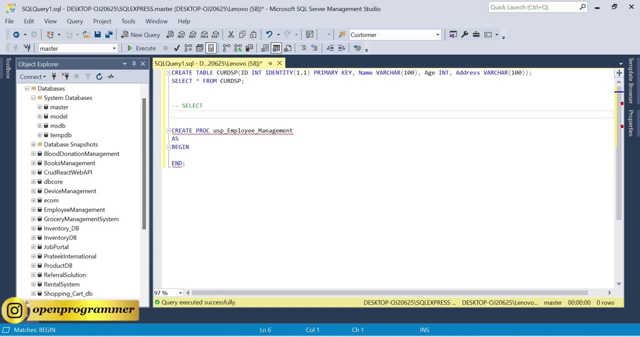 Your Select, Select The Select, The Select, Update and delete. So what, Basically, we can do? if you want, we can create four stored procedures respective to each operation: one for select, one for insert, one for update, one for delete. but instead of creating, for You know, stored procedures, 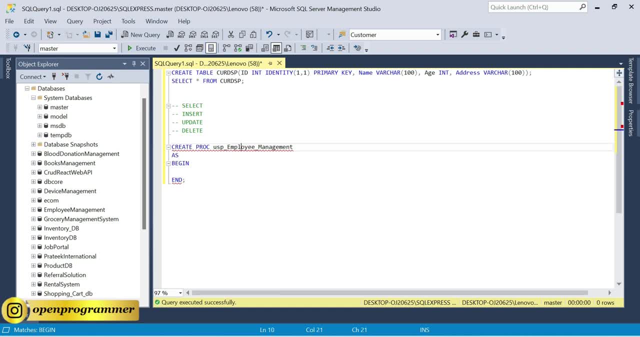 we can create a simple one, stored procedures and based on a flag, or you can say based on a type we can differentiate for which block it should execute it. all right, let me show you how we can do that. first of all, let's add some variables. so the first is id, int and the name we are going to. 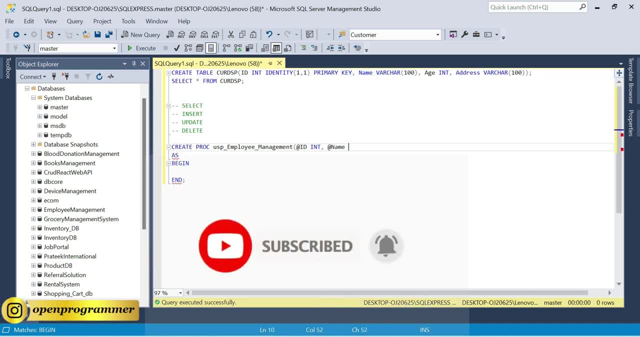 use the same. you know variables for the stored procedure, let's copy and paste it over here and use at the rate of with every variable. so for this stored procedure we are having four variables: I d name, age, address and last one is type. so where care hundred? so now, if here, let me check if at the 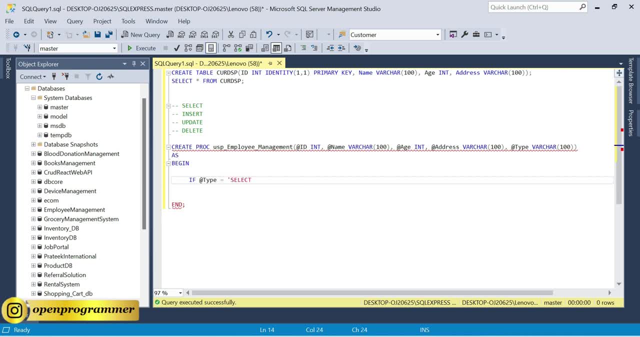 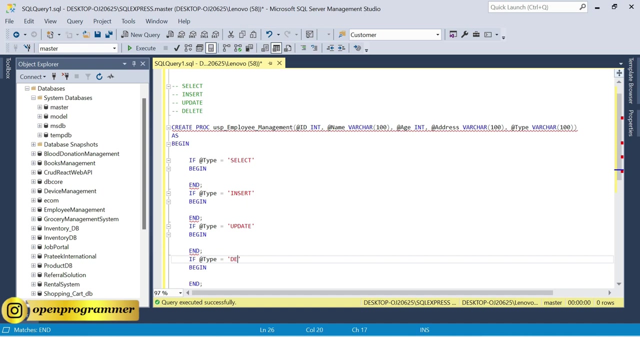 rate type equal: select, then it will go to this block. begin, and so let me copy this and paste: if the type is insert, then it goes to this block, and if type is update, so it will go to this block. and finally, if the type is delete, then it goes to this block. so, simply for the select, copy this command and 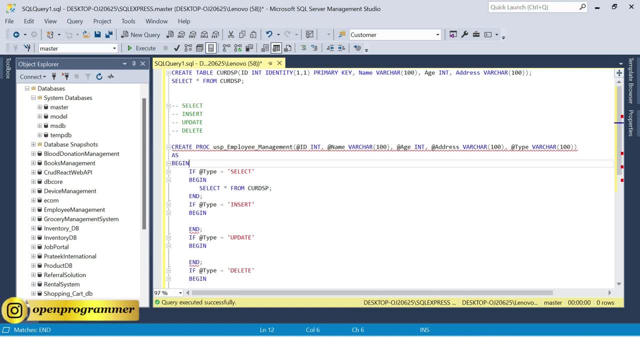 paste it over here. so if I pass type select, then it goes to this block. it is skipped, these three blocks, all right. and if we type insert, then it goes to this block. so let's write the command: so insert into the table name. sorry, I misspelled this. so name age. 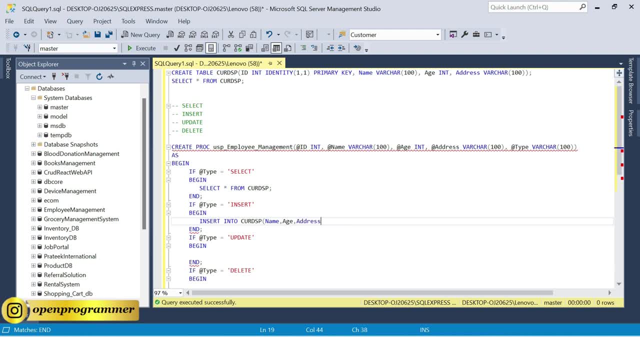 address values. so if your new to SQL server then your negative. an equal business video in my channel of the basics, to start with, equals over. so and if you use his used the name will use age for addresses. you use address, alright. so this is how all can insert data through a type. so if we come to the updates, so let's update the. 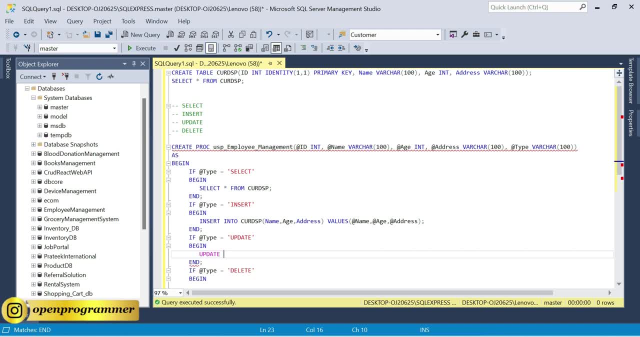 table. so update the table name. table name is this: and then set: set name equal to at the rate name, age equal at the rate age and address is equal to address where ID is equal to at the rate ID. so whatever ID we will pass, it will go to: 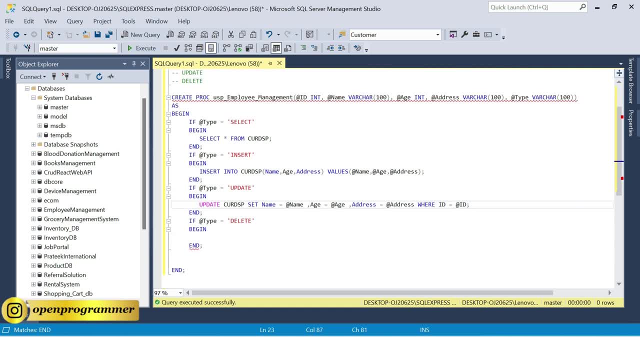 the table and today the respective records. now comes to the delete part. so here delete from the table name where we will pass id. so based on id, we will delete that particular record id. so we are done with our stored procedure. so let's select this complete block and execute. 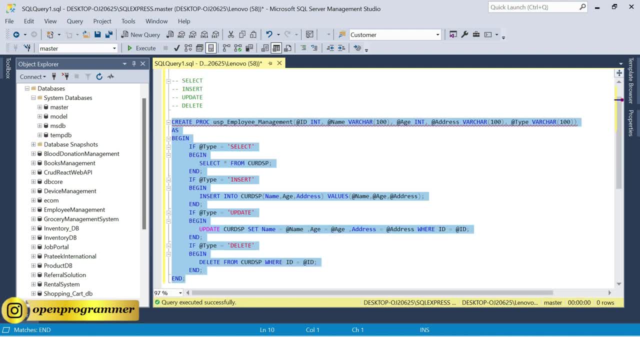 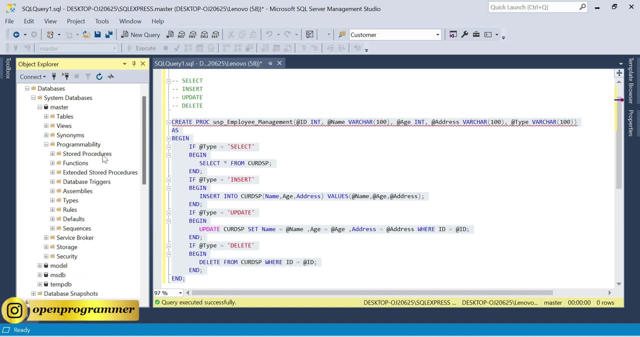 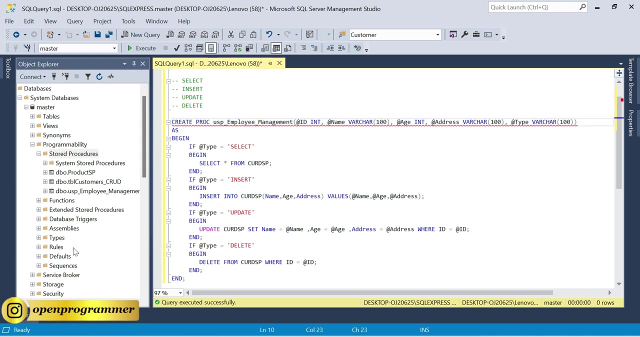 you can see command completed successfully. so we, if you go to your master database and go to your programmability- and here we have a separate section for stored procedures- if you expand that right click on this stored procedure and refresh so you can see usb employee management. here you can see that usb employee management and we expand this. 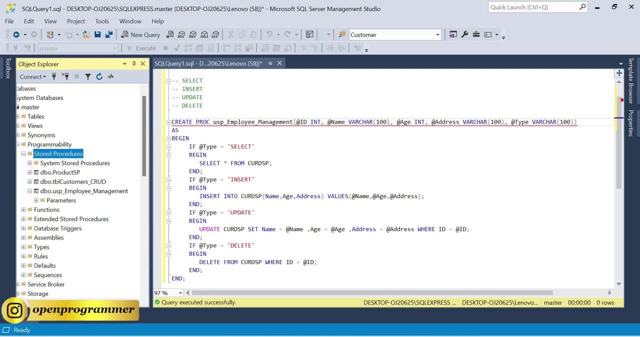 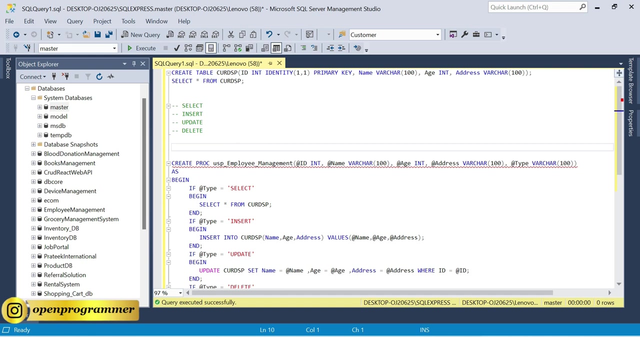 so it will show you all these parameters. id name, age. so there is a block for parameters. expand this. you can see id name, age, address type. you can see these five variables are available here. so let me close this so now. so we have created our stored procedure. now let's try to call it. 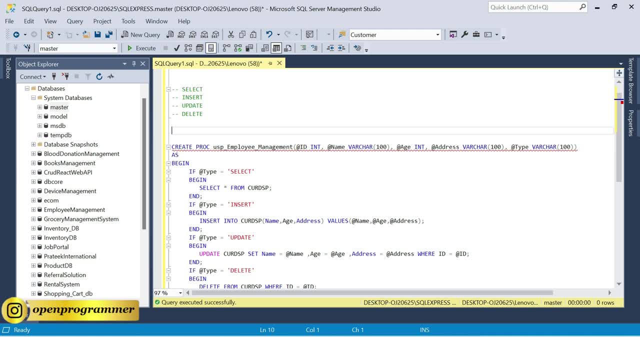 so to execute uh, or to call a store procedure, we will use e, x, e, c, that is a short form- execute, execute then the procedure name and then we need to give the values of these respective variables. so first we will call this select block, so for select. 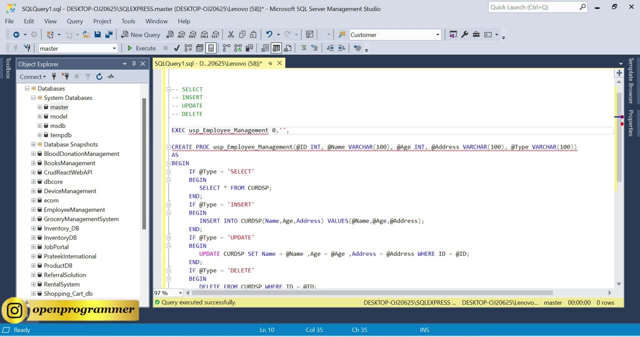 id should be zero and name is blank. age is blank, not blank zero, because we have used integer for this age variable and address all the Vielen: eight plus eight nul, nul, nul nul. if you want b too nul nul, then you put in h column u, click on this eat file. let me relax one and that will allow you to convert the item itself. so let's retail thisご確 forgot that we don't want additional return. 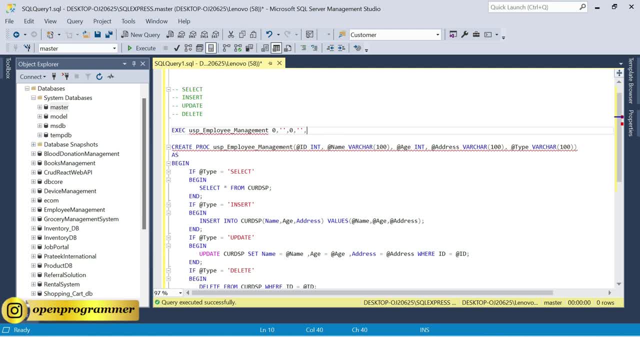 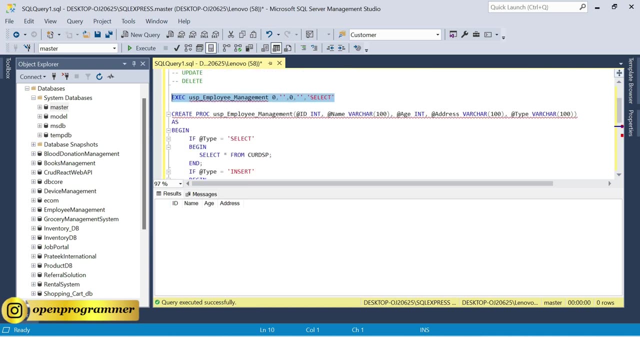 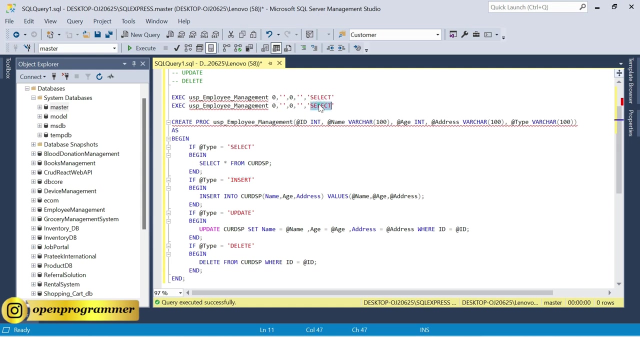 for this age variable and address also blank, and then type should be select. so if i execute this command, so you can see we got a blank table because as of now there is no record. all right, so now let me copy this same, paste it over here. now we will use this insert command, so for that, 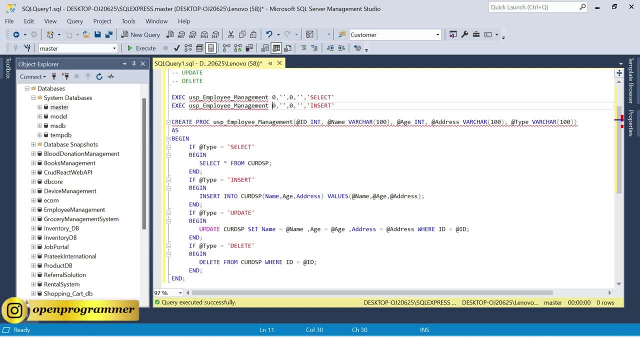 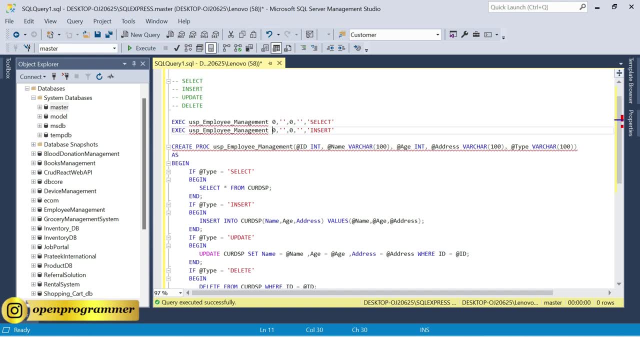 insert. we don't. we don't need to pass any id column because we already use int identity, so it automatically create a id column or id value. so for name, let me give my name, and for age, let me give my age. that is not correct one. and for address, let's say india. 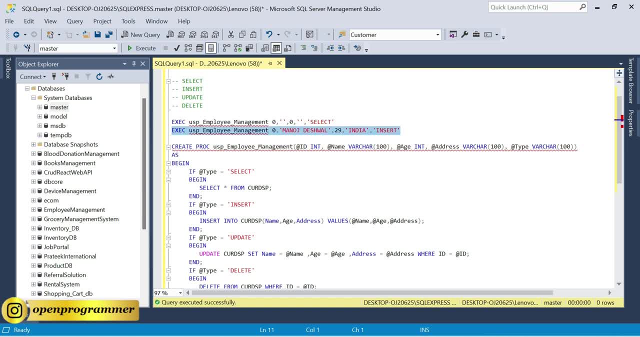 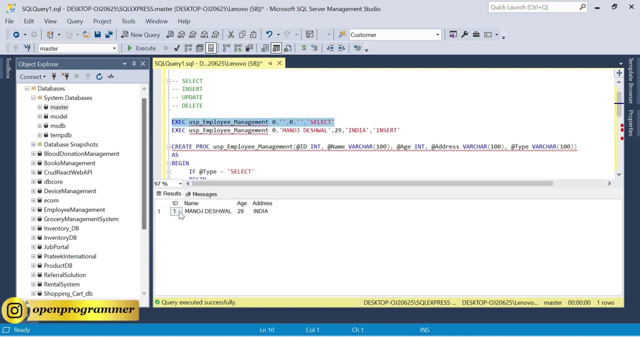 and type is insert. if i select this command and execute, you can see one row affected, and if i try to execute the select. so now we are getting one value, perfect. let me also add another value. so we now we have two rows in our table, perfect. so now we will use our update block. so let's copy. 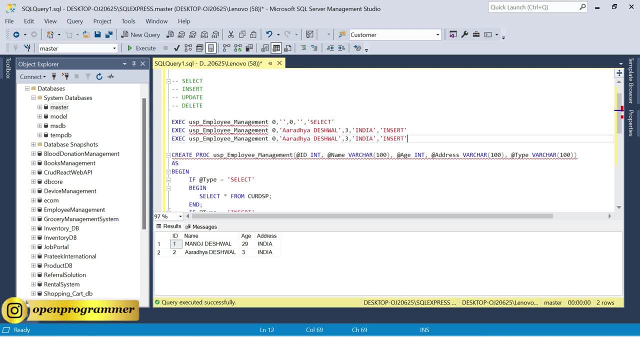 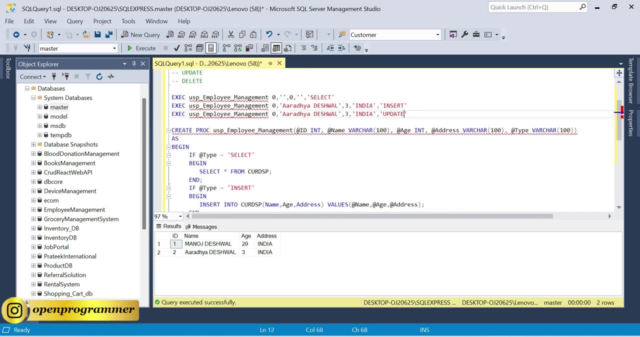 this command and paste it over here and change the type. copy and paste. so let's say we need we, we want to change this name and this age, all right. or let's say we need to change everything: name, age, india, how we can do that. so let's say we want to change name from aradya deshwal to aradya only. 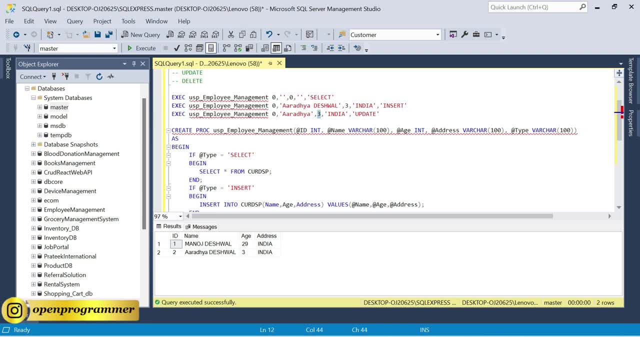 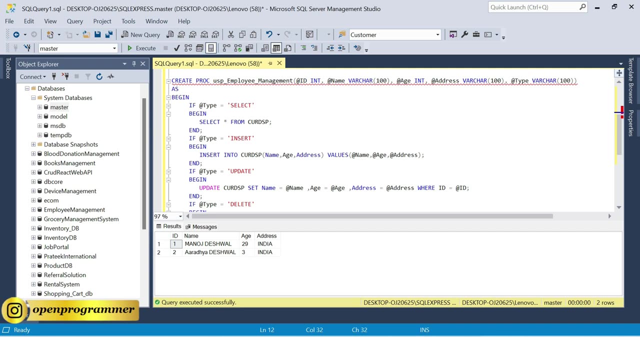 so let's give her the correct name and let's say age is two, and here let's say hariana, india. all right, so select this command and here we need to pass a already passed id and based on this id value, it will search to this entire table and whenever it. 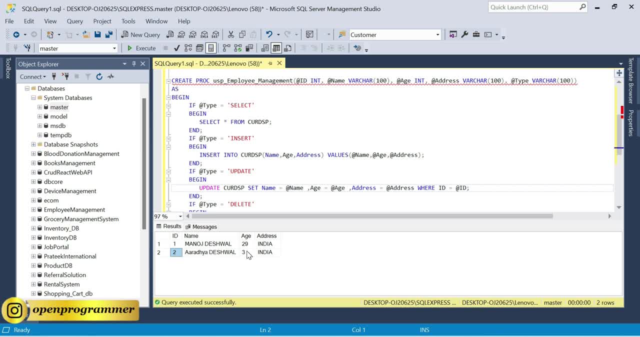 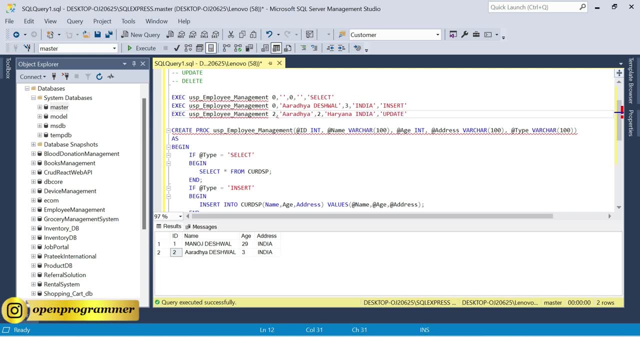 matches with the id value, it goes to that particular record and update all the values. so for this we need to pass id. so aradya's id is two, so let's pass this two and let me change age to five. so select this command and execute so you can see one row affected, if I 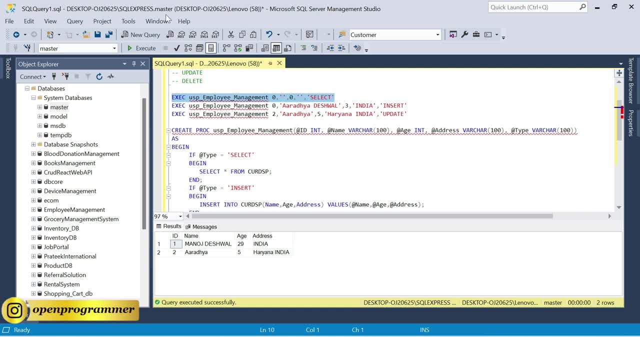 again. select the records so you can see the values. has been changed from aradya deshwal to aradya, age three to five. address india to hariana india. so this, that is how you can use your update command. all right, so let's also add another row and select your. 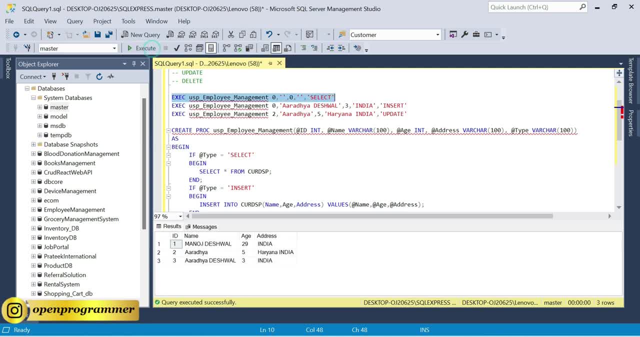 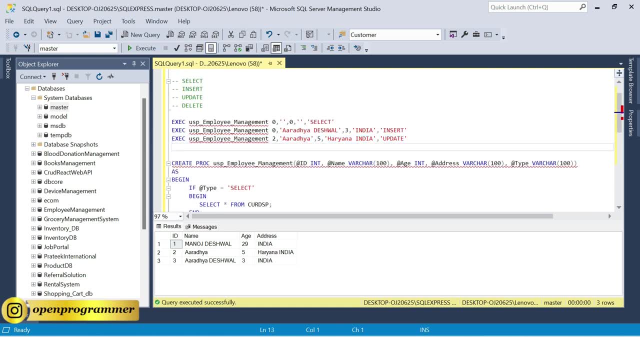 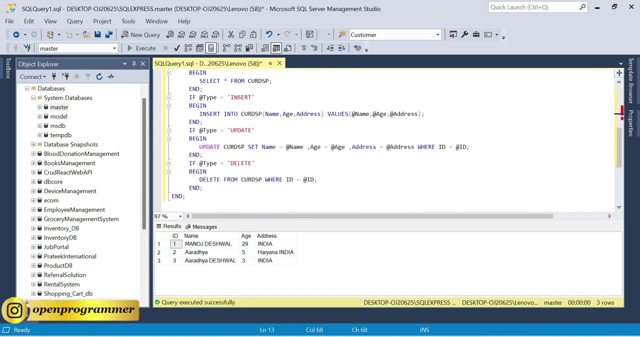 entire table. so as of now we have three rows. all right, so now the last operation is delete. how we can do that? so select, copy this command and paste and copy this delete if you go to that section. so for delete we only need id, nothing else. so let's say: 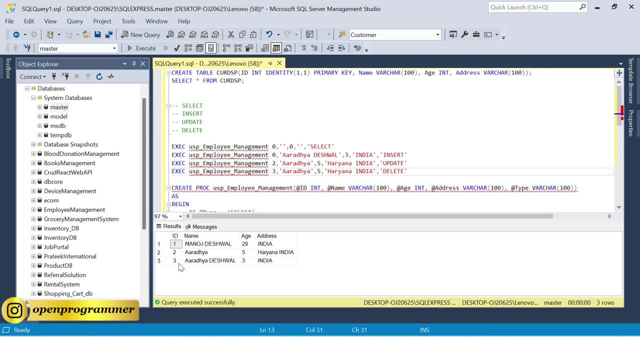 if we want to delete that third row with the id value three. so we don't need name value, we don't need age you, we don't either need address, but we need id and type. so select this command, execute so you can see one row factored if you again go to the select. 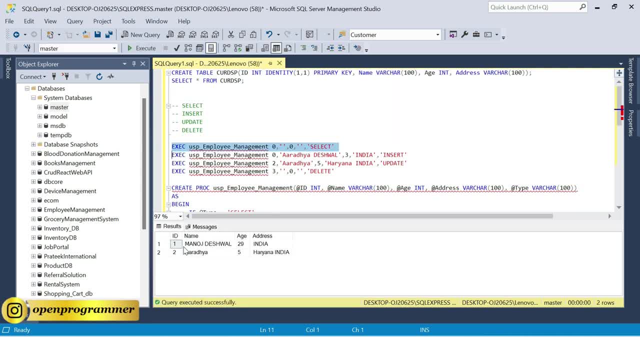 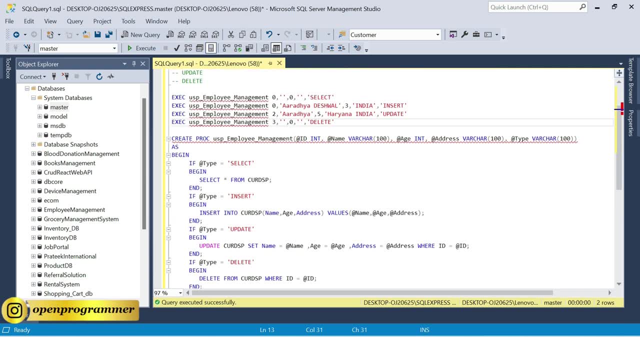 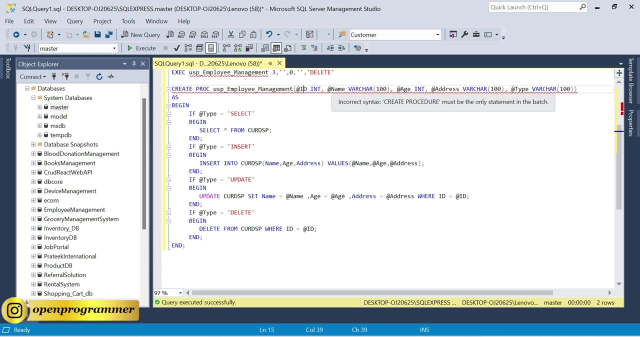 command and execute so you can see that row with the id3 has been deleted. perfect, so this is how you can simply create your stored procedures. obviously, for your particular requirement or project details, you should have different kind of variables over there, but these are the basic operations which you can perform using this same pattern, same format. all right, so this is about. 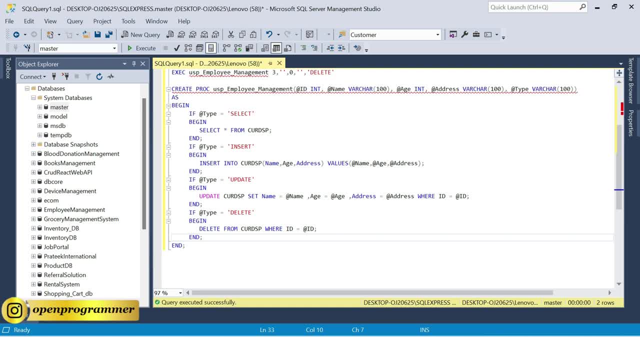 today's video if you like it. if you did so, hit the like button, share, comment and if you are facing any problem, difficulty in your project or in your assignment, so you can connect with me on my instagram. my instagram handle is open programmer. you can also email me your queries. 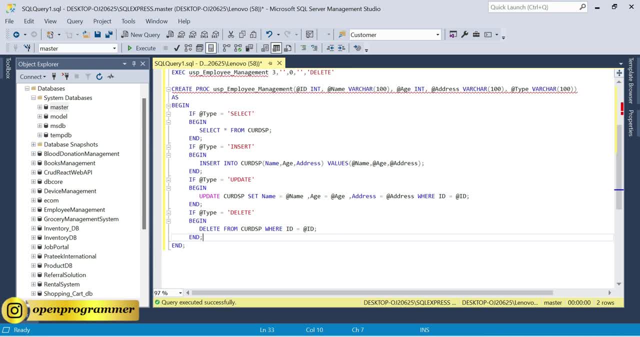 so you can find both the contact details in my channel description. i basically do the paid services for interns and college students, so you can connect with me for any kind of your query. regarding react js, you know a java script: jquery, sql server c, sharp mvc web api, so for sure we'll. 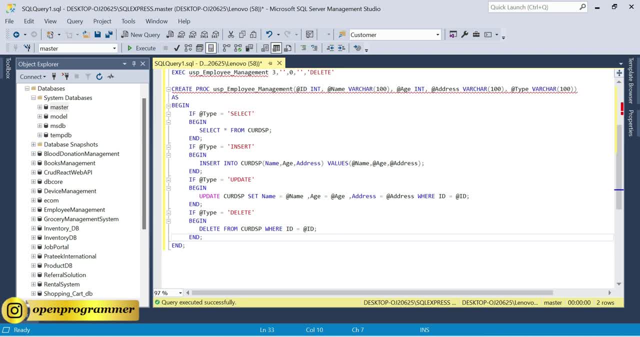 connect and help each other. so i'll see you in the next one. thanks for watching. take care, bye.